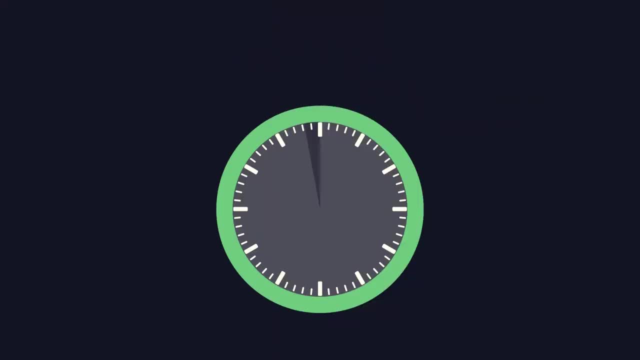 For example, if you were to say a 57-minute journey would take about an hour, you would be approximating A value can be approximated by rounding, usually to a value that is easier to work with. Be aware: for approximation questions you are rarely allowed a calculator. 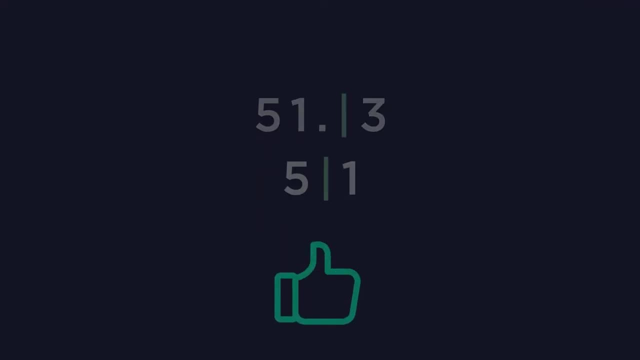 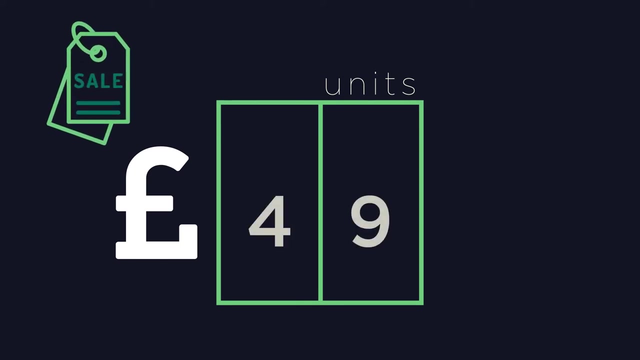 A good rule of thumb for approximating is to round to a position that is one or two positions above the lowest position of the original value. Let's see an example of this rule in action. Say you are purchasing something that's £49.. The lowest positional value is 9, in the Units. 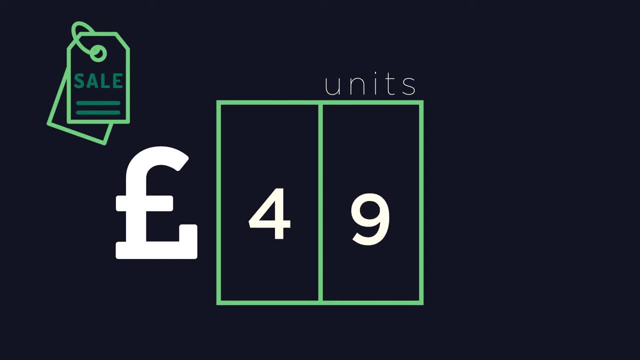 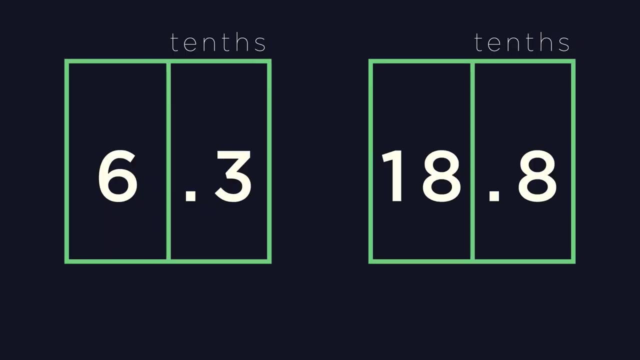 column. Using our rule, we round to one position higher, which gives us £50.. Because 50 is a multiple of 10, it's a much easier value to work with. so our approximation is £50.. Let's go on to approximating these questions, rounding it up just one place: value Pause. 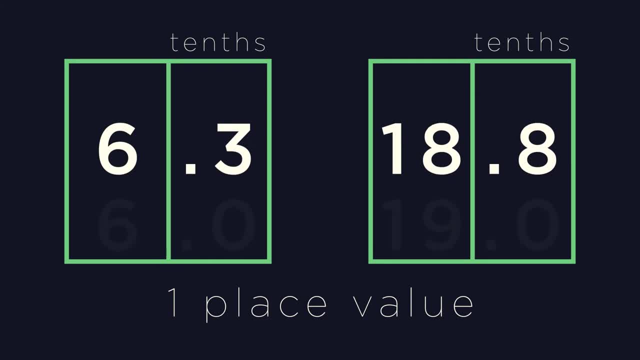 and have a try. How did you do? If we look at 6.3,, its lowest positional value is 3, in the Tenths column, so we round it up one position to just 6.. For 18.8, the lowest positional value is 8, in the Tenths column, so we would round up. 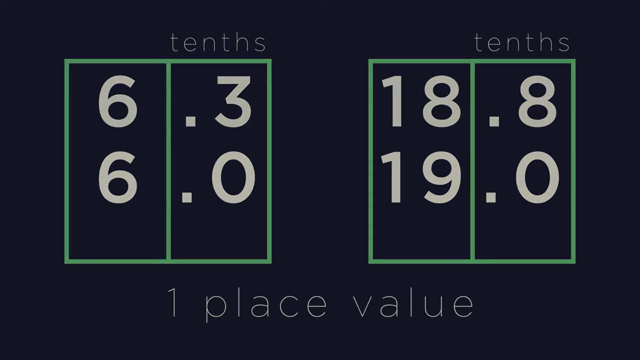 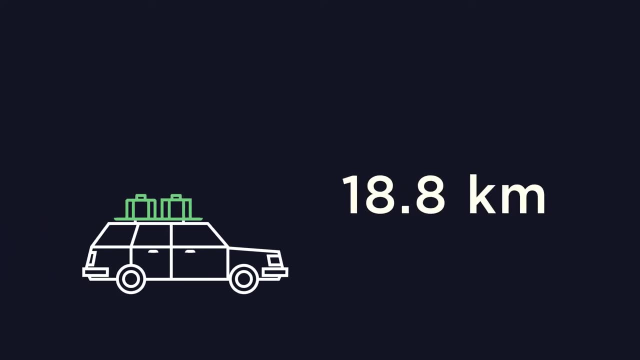 giving us an approximation of 19.. However, if we add some context, let's say you are going on a journey that is 18.8 kilometres. You're trying to calculate the time it will take and are happy to approximate, You know. 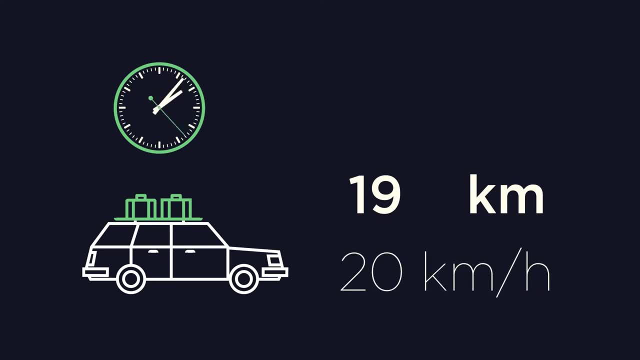 you can travel at 20 kilometres per hour. Whilst it's certainly possible to calculate time from these values, looking at your approximated distance- 19 kilometres- it is still not the easiest value to work with At this stage. we can therefore approximate a second time. What do you think that would? 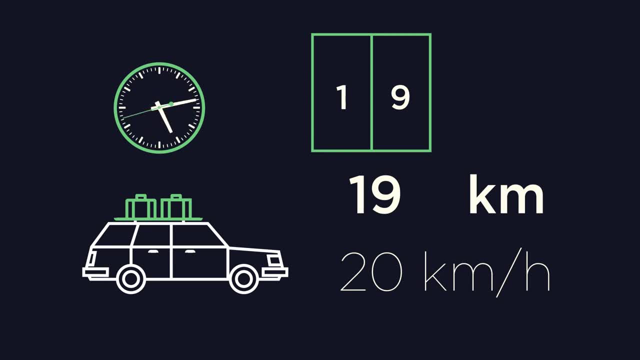 give us. If we look at the 9 as the lowest possible value positionally, it would round upwards making the 10 a 20.. Now, if we look at our values, we have a distance of 20 kilometres, a speed of 20 kilometres per hour and, using distance over speed, we get a time of 1 hour.